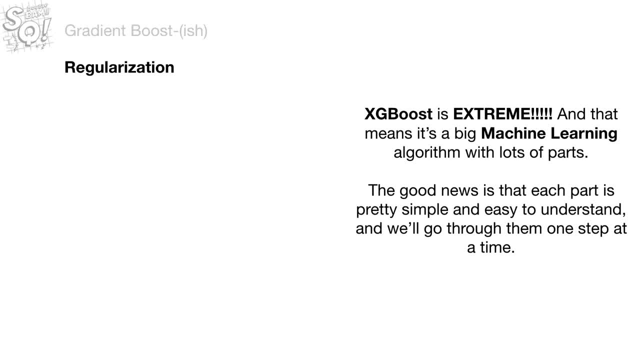 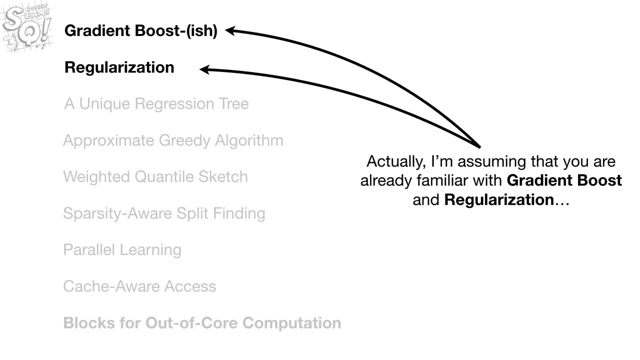 XGBoost is extreme and that means it's a big machine learning algorithm with lots of parts. The good news is that each part is pretty simple and easy to understand, and we'll go through them one step at a time. Actually, I'm assuming that you are already familiar with Gradient Boost and regularization. 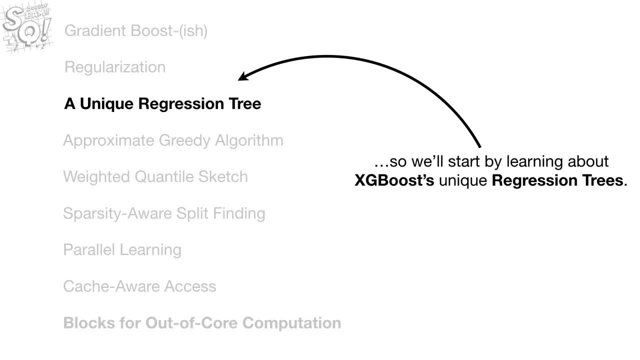 So we'll start by learning about XGBoost's unique regression trees. Because this is a big topic, we'll spend three whole StatQuests on it. In this StatQuest, we'll learn about the XGBoost tree and we'll learn about the XGBoost tree. 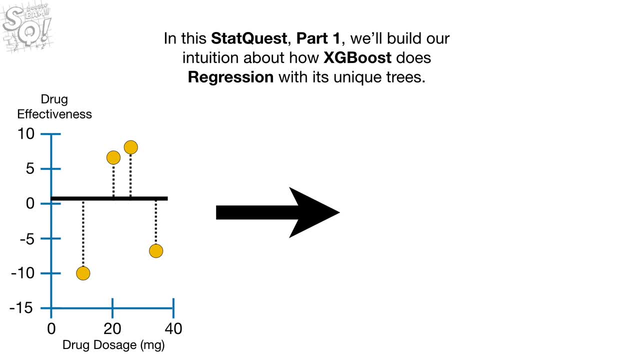 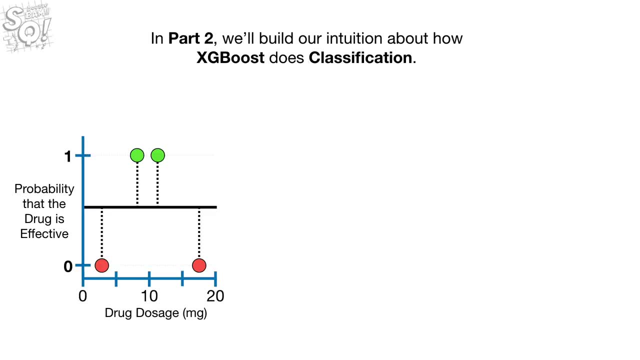 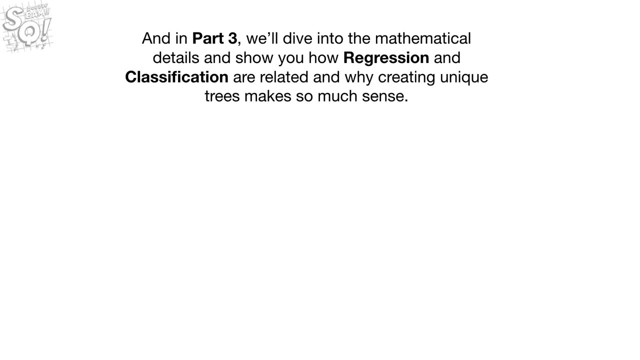 In this StatQuest- Part 1, we'll build our intuition about how XGBoost does regression with its unique trees. In Part 2, we'll build our intuition about how XGBoost does classification. And in Part 3, we'll dive into the mathematical details and show you how regression and classification are related. 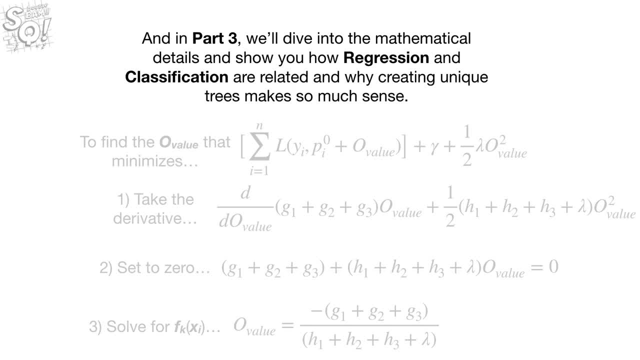 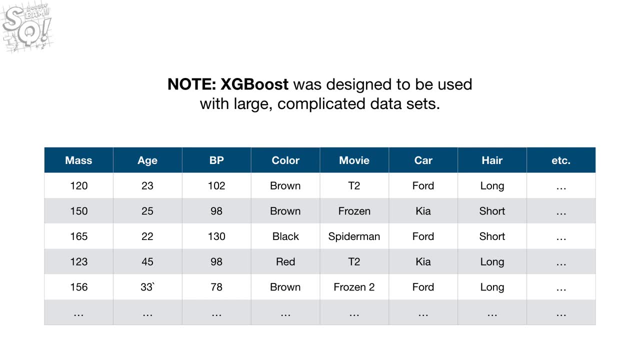 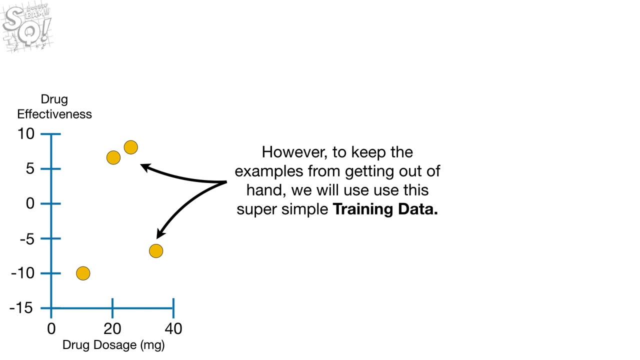 and why creating unique trees makes so much sense. Note: XGBoost was designed to be used with large, complicated data sets. However, to keep the examples from getting out of hand, we'll use this super simple training data. On the x-axis, we have different drug dosages. 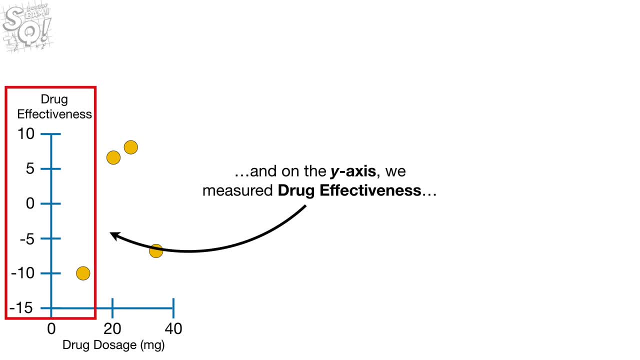 And on the y-axis we've measured drug effectiveness. These two observations have relatively large positive values for drug effectiveness, and that means that the drug was helpful. These two observations have relatively large negative values for drug effectiveness, and that means that the drug did more harm than good. 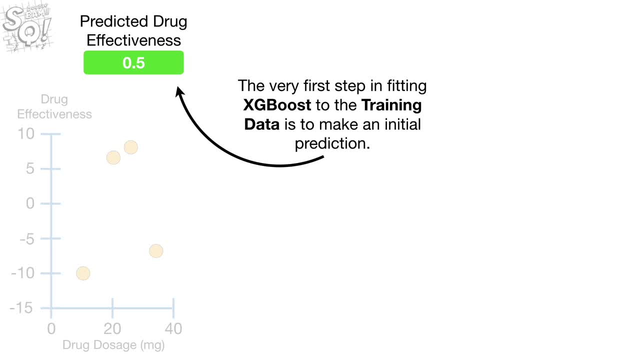 The very first step in fitting XGBoost to the training data is to make an initial prediction. This prediction can be anything, but by default it is 0.5, regardless of whether you're using XGBoost for regression or classification. 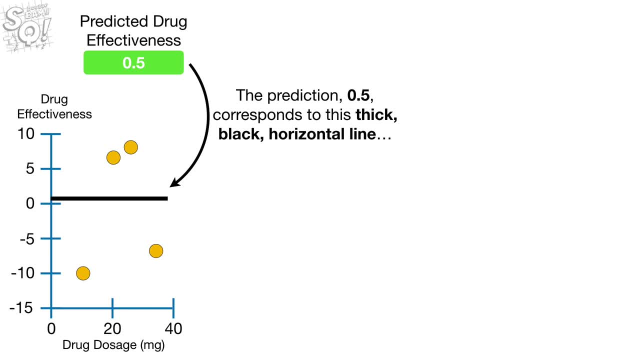 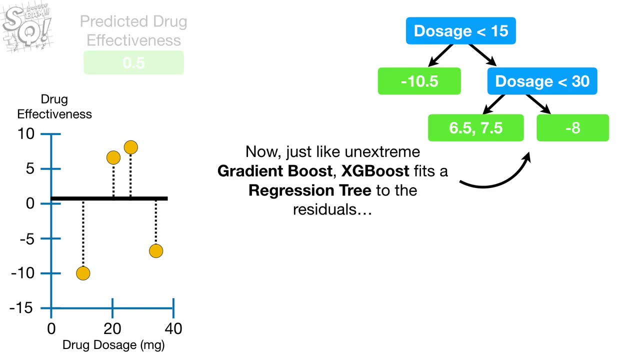 The prediction 0.5, corresponds to this thick black horizontal line And the residuals. the differences between the observed and predicted values show us how good the initial prediction is. Now, just like Unextreme Gradient Boost, XGBoost fits a regression tree to the residuals. 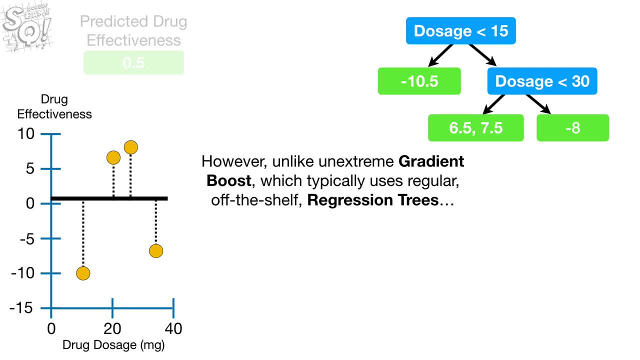 However. However, Unlike Unextreme Gradient Boost, XGBoost fits a regression tree to the residuals. Unlike Unextreme Gradient Boost, which typically uses regular off-the-shelf regression trees, XGBoost uses a unique regression tree that I call an XGBoost tree. 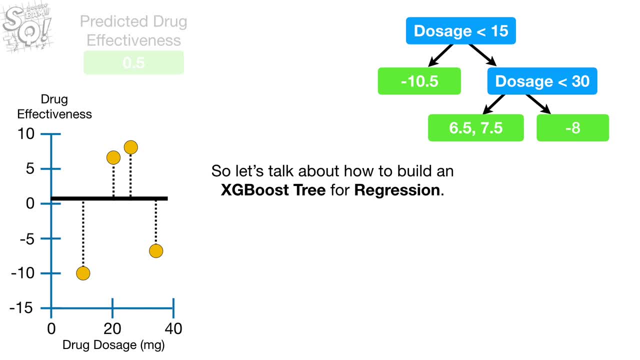 So let's talk about how to build an XGBoost tree for regression. There are many ways to build XGBoost trees. This video focuses on the most common way to build them for regression. Each tree starts out as a single leaf. Each tree starts out as a single leaf. 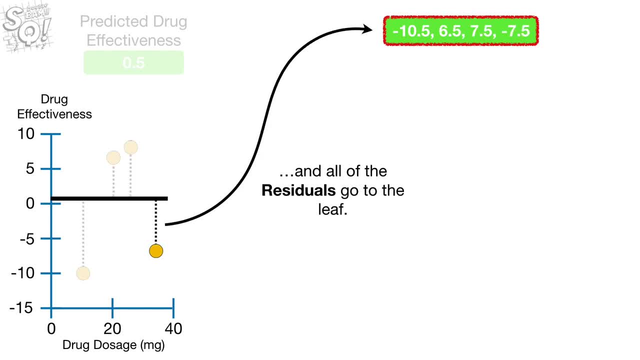 And all of the residuals go to the leaf. Now we calculate a quality score or similarity score for the residuals. The similarity score equals the sum of the residuals squared over the number of residuals plus lambda. Note: lambda is a regularization point. 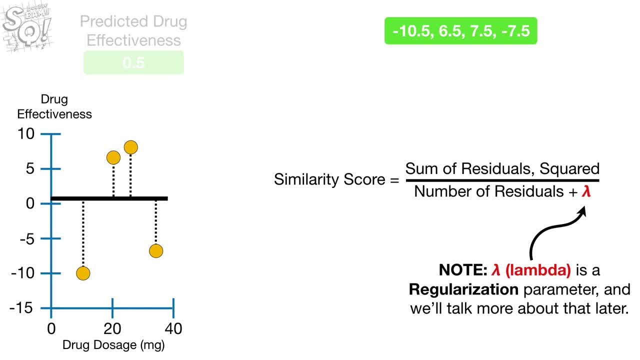 Note: lambda is a regularization point. Note: lambda is a regularization point parameter and we'll talk more about that later. For now, let lambda equals 0. Now we plug the four residuals into the numerator and since there are four residuals in the leaf, we put a 4. 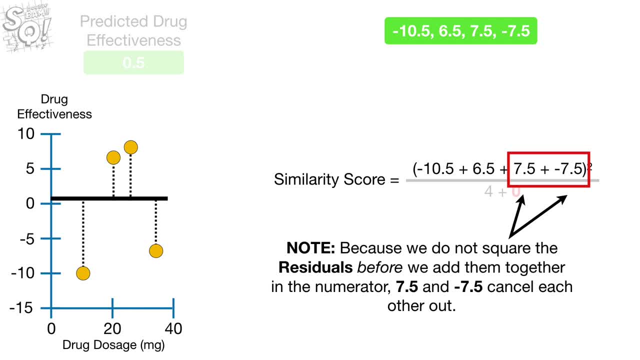 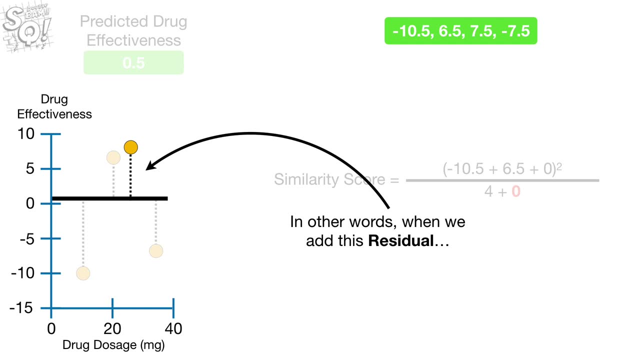 in the denominator Note because we do not square the residuals before we add them together in the numerator. 7.5 and negative 7.5 cancel each other out. In other words, when we add this residual to this residual, they cancel each other out. Likewise, 6.5 cancels out most of negative 10.5,. 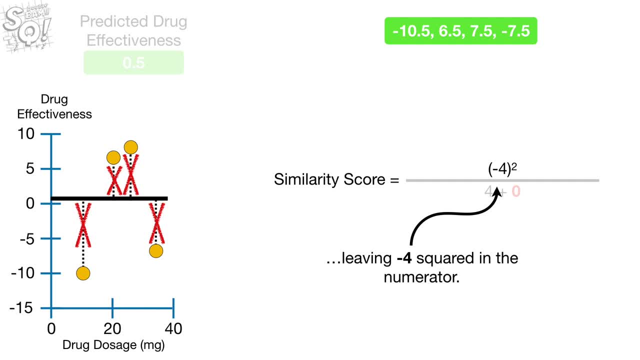 leaving negative 4 squared in the numerator. Thus the similarity score for the residuals, the root, equals 4.. So let's put similarity equals 4 up here so we can keep track of it. Now the question is whether or not we can do a better job clustering similar residuals. 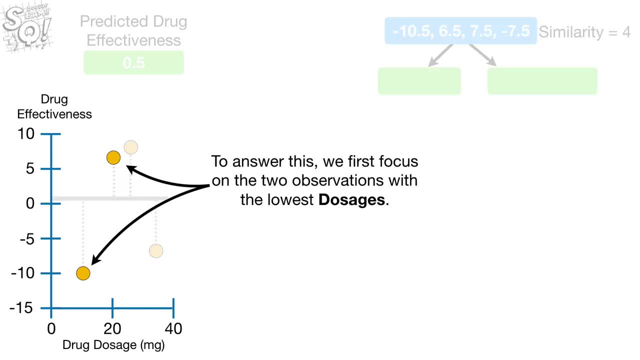 if we split them into two groups. To answer this, we first focus on the two observations with the lowest dosages. Their average dosage is 15, and that corresponds to this dotted red line. So we split the observations into two groups based on whether or not the dosage is less than 15.. 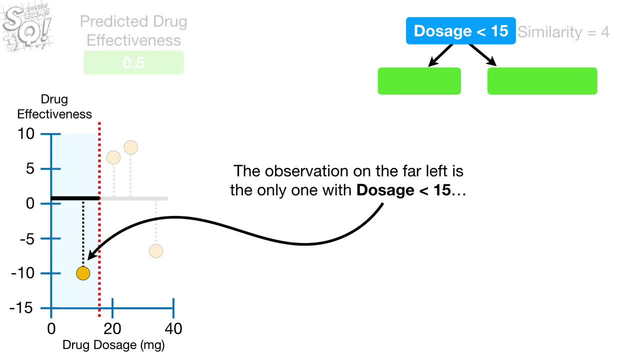 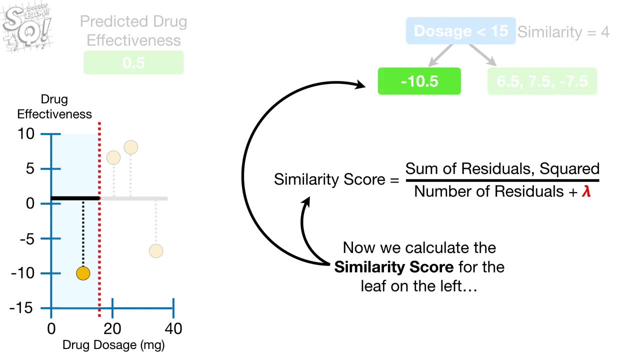 The observation on the far left is the only one with dosage less than 15, so its residual goes to the leaf on the left. All of the other residuals are the same. All of the other residuals go to the leaf on the right. Now we calculate the similarity score for the leaf on the left. 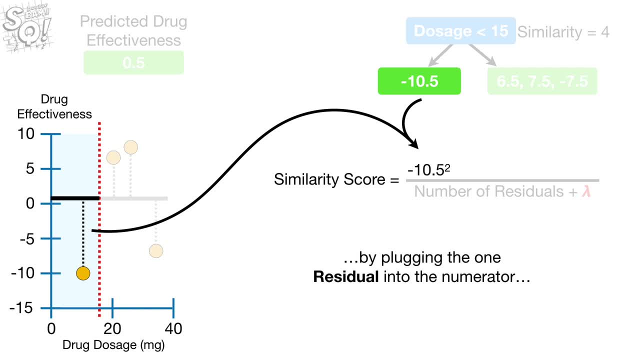 by plugging the one residual into the numerator. and since only one residual went to the leaf on the left, the number of residuals equals 1.. And, just like before, we set lambda equal to 0, and the similarity score for the leaf on the left. 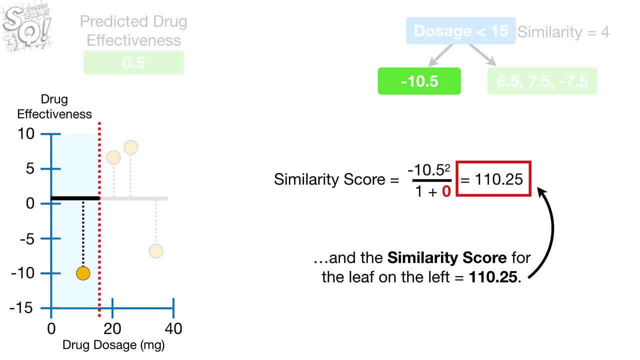 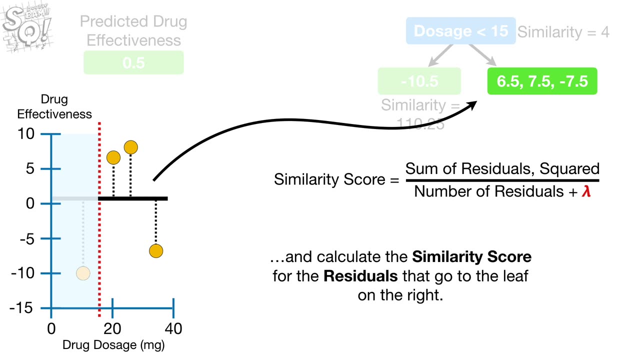 equals 110.5.. So let's put similarity equals 110.25 under the leaf so we can keep track of it and calculate the similarity score. for the residuals that go to the leaf on the right, We plug in the sum of residuals squared into the numerator. 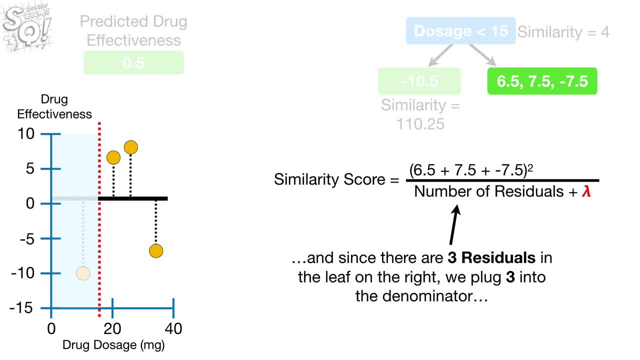 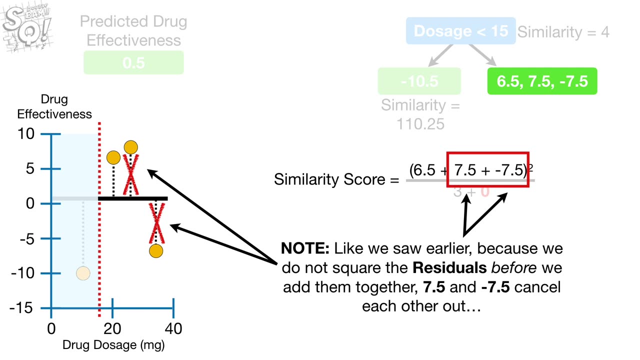 and since there are 3 residuals in the leaf on the right, we plug 3 into the denominator and check the weight Just like before. let's let lambda equals 0.. Like we saw earlier, because we do not square the residuals before we add them together. 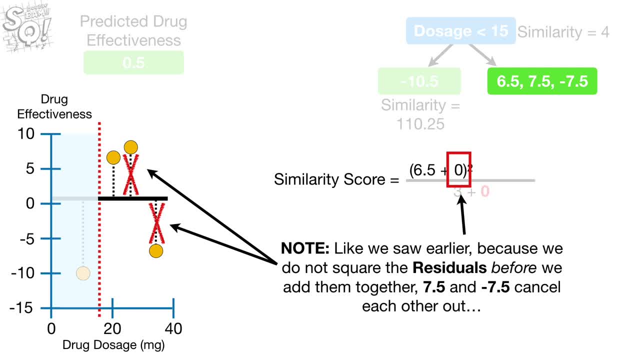 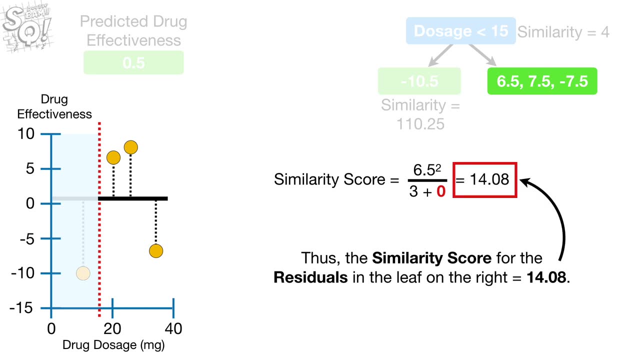 7.5 and negative 7.5 cancel each other out, leaving only one residual- 6.5, in the numerator. Thus the similarity score for the residuals in the leaf on the right equals 14.08.. So let's put similarity equals 14.08 under the leaf so we can keep track of it. 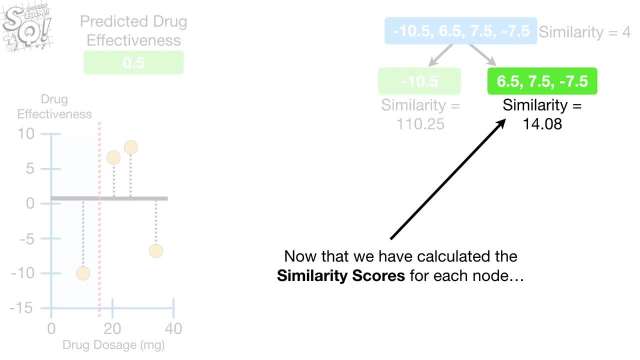 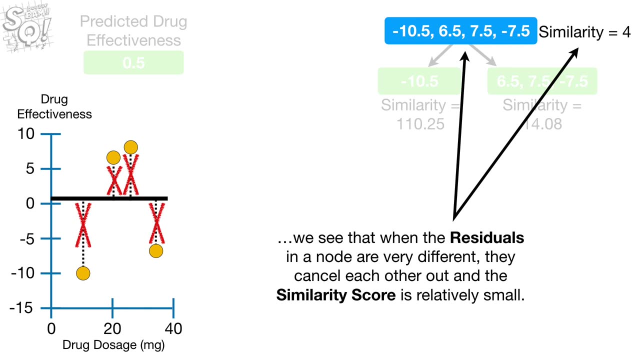 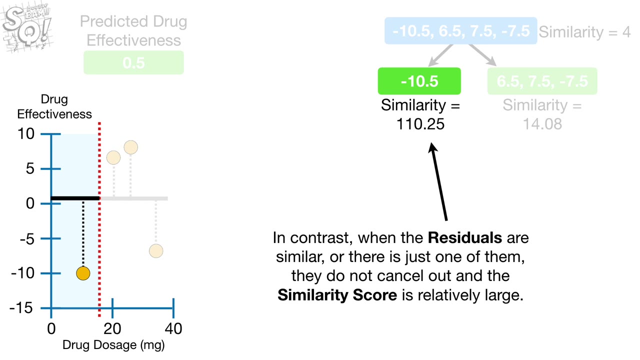 Now that we have calculated similarity scores for each node, we see that when the residuals in a node are very different, they cancel each other out and the similarity score is relatively small. In contrast, when the residuals are similar or there is just one of them, 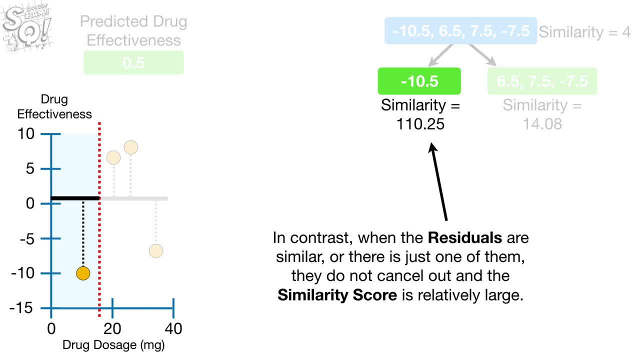 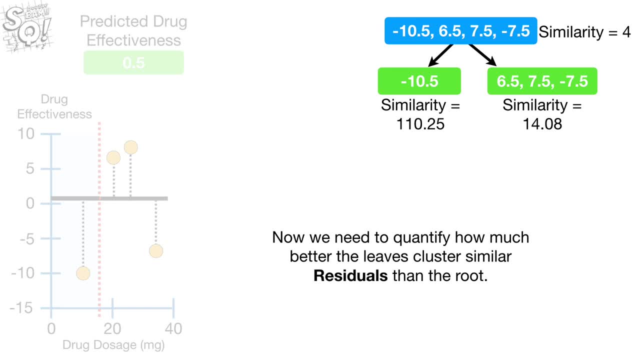 they do not cancel out and the similarity score is relatively large. Now we need to quantify how much better the leaves cluster similar residuals than the root. We do this by calculating the gain of splitting the residuals into two groups. Gain is equal to the similarity score for each node. 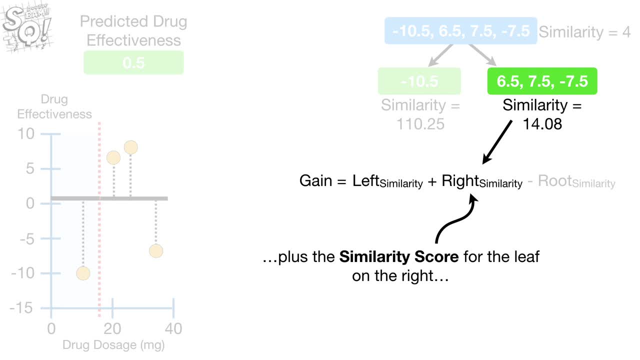 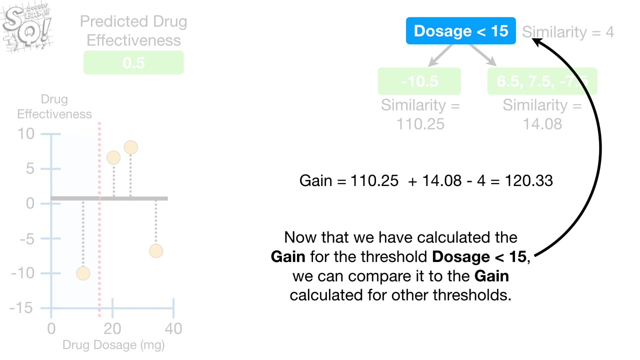 The similarity score for the leaf on the left plus the similarity score for the leaf on the right, minus the similarity score for the root. Plugging in the numbers gives us 120.33.. Small bam, Now that we have calculated the gain for the threshold of dosage, less than 15,. 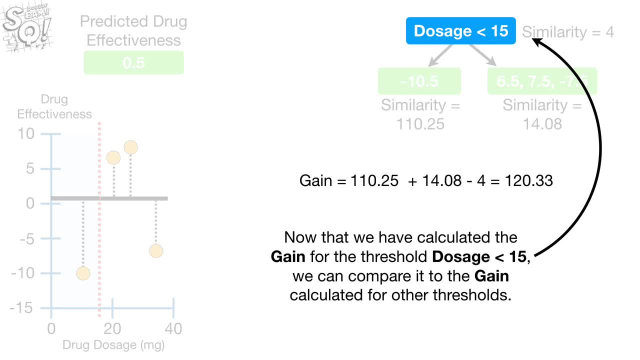 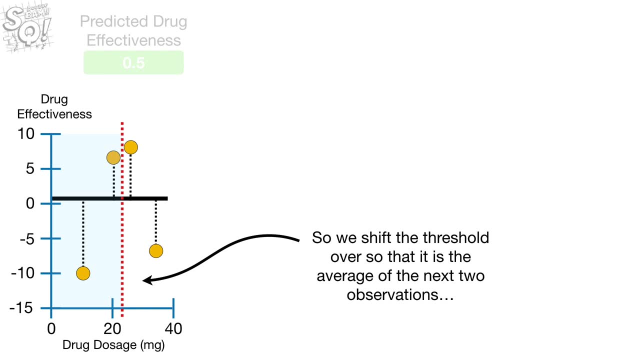 we can compare it to the gain calculated for other thresholds. So we shift the threshold over so that it is the average of the next two observations and build a simple tree that divides the observations using the new threshold dosage less than 22.5.. 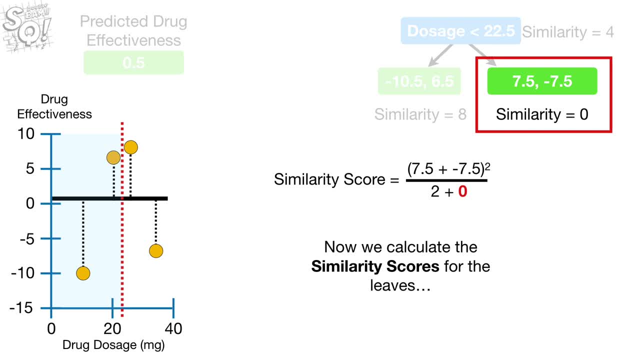 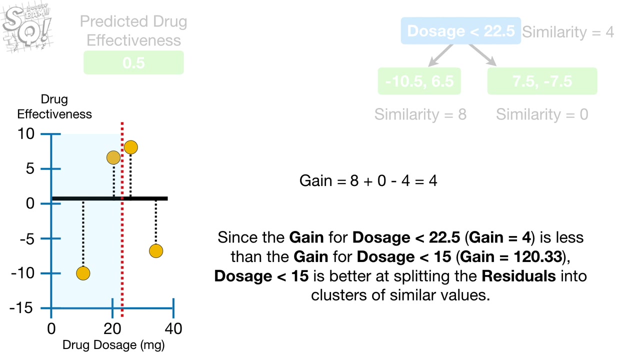 Now we calculate the similarity scores for the leaves and calculate the gain. The gain for dosage less than 22.5 is 4.. Since the gain for dosage less than 22.5 is less than the gain for dosage less than 15,, 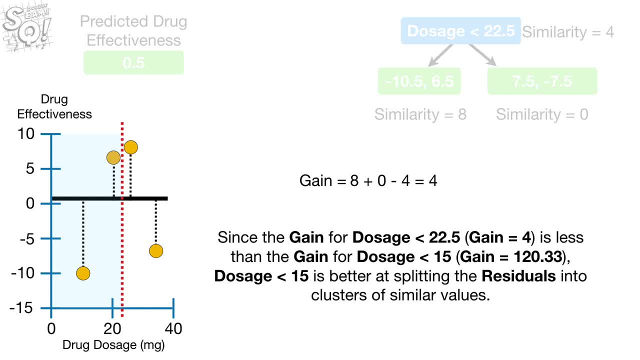 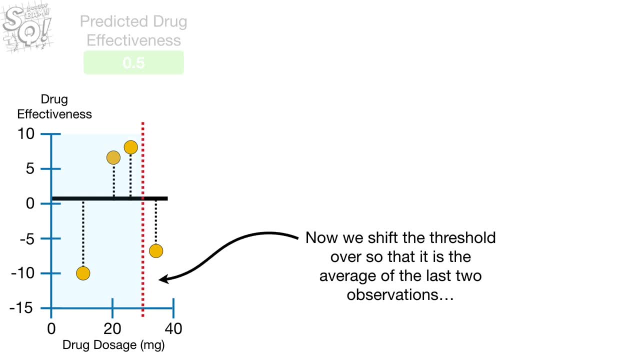 dosage less than 15 is better at splitting the residuals into clusters of similar values. Now we shift the threshold over so that it is the average of the last two observations and build a simple tree that divides the observations, using the new threshold dosage less than 30.. 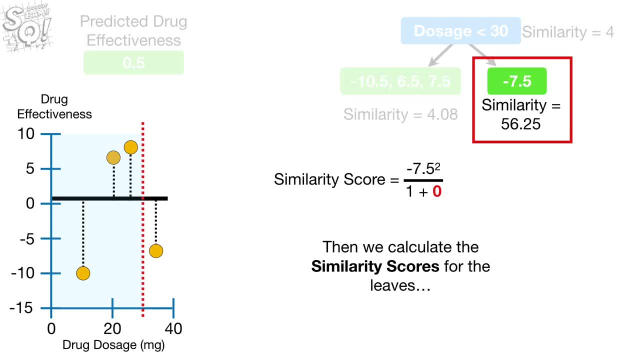 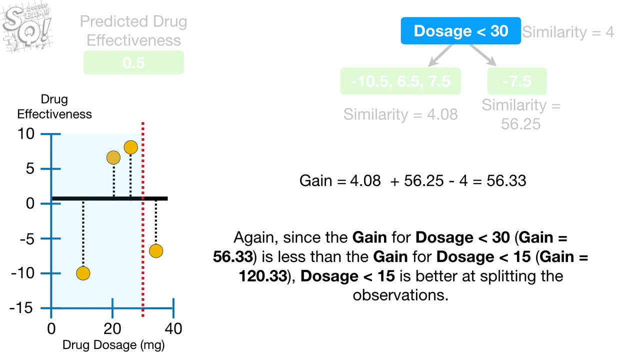 Then we calculate the similarity scores for the leaves and the gain. The gain for dosage less than 30 equals 56.33.. Again, since the gain for dosage less than 30 is less than the gain for dosage less than 15, dosage less than 15 is better at splitting the observations. 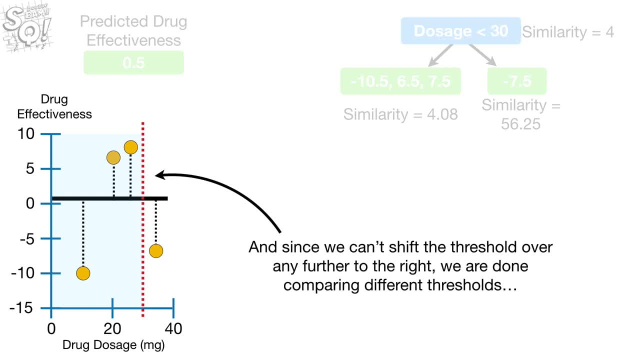 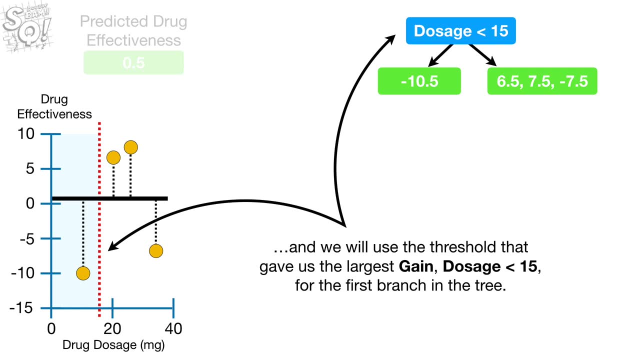 And since we can't shift the threshold over any further to the right, we are done comparing different thresholds And we will use the threshold that gave us the largest gain dosage- less than 15, for the first branch in the tree Now, since there is only one residual in the leaf on the left, 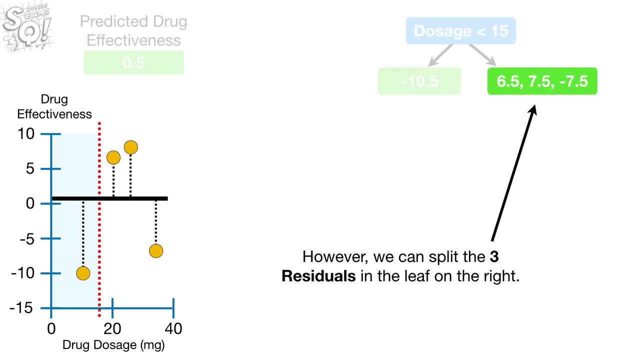 we can't split it any further. However, we can split the three residuals in the leaf on the right. So we start with these two observations and their average dosage is 22.5, which corresponds to this dotted green line. So the first threshold that we try is dosage less than 22.5.. 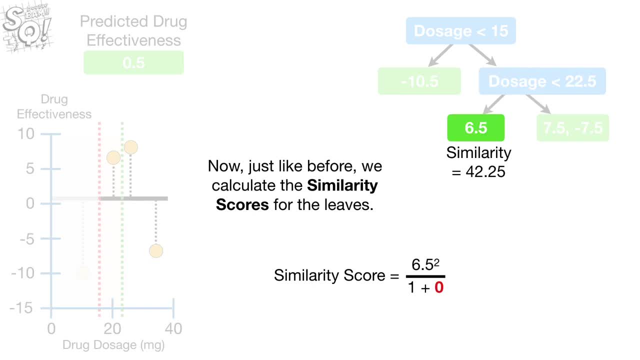 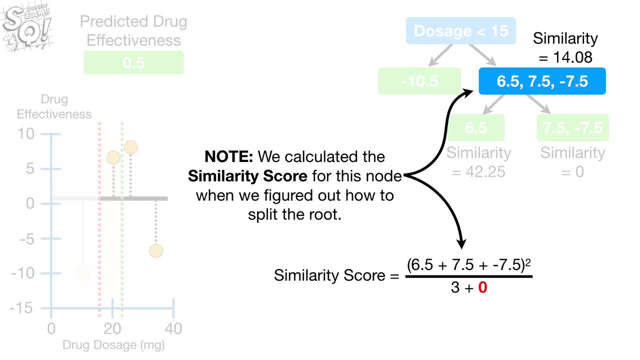 Now, just like before, we calculate the similarity scores for the leaves. we calculated the similarity score for this node when we figured out how to split the root, So now we calculate the gain And we get. gain equals 28.17 for when the threshold is dosage less than 22.5.. 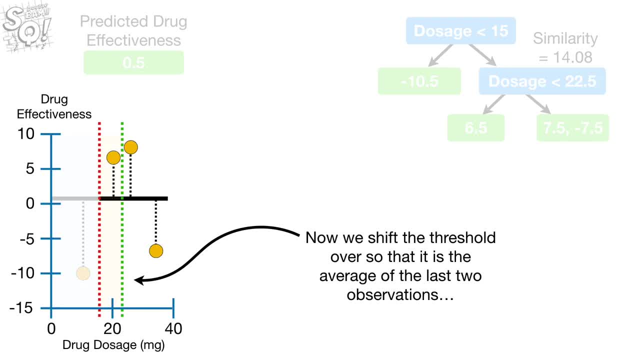 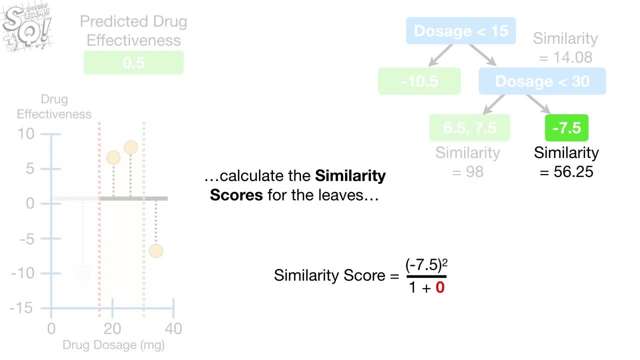 Now we shift the threshold over so that it is the average of the last two observations. calculate the similarity scores for the leaves and the gain And we get. gain equals 28.17 for when the threshold is dosage less than 22.5.. 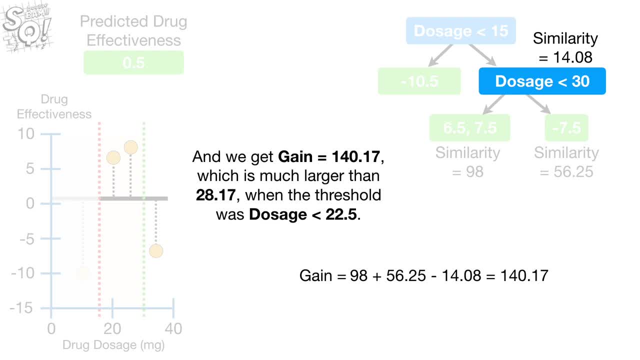 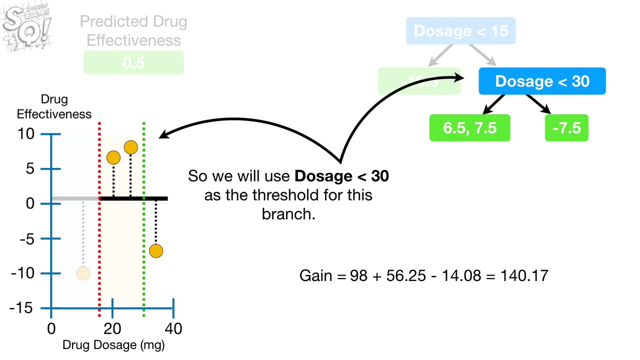 And we get gain equals 140.17, which is much larger than 28.17 when the threshold was dosage less than 22.5.. So we will use dosage less than 30 as the threshold for this branch to keep this example from getting out of hand. 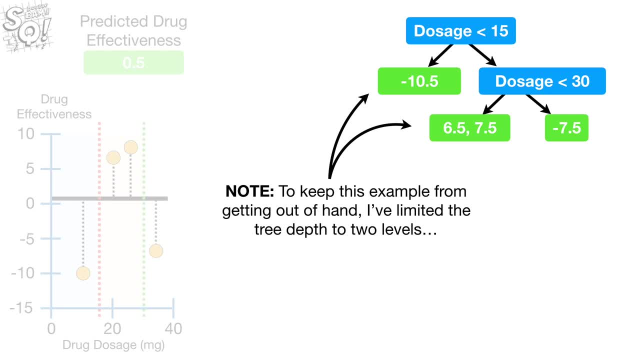 I've limited the tree depth to two levels And this means we will not split this leaf any further and we are done building this tree. However, the default is to allow up to six levels Small bam. Now we need to talk about how to prune this tree. 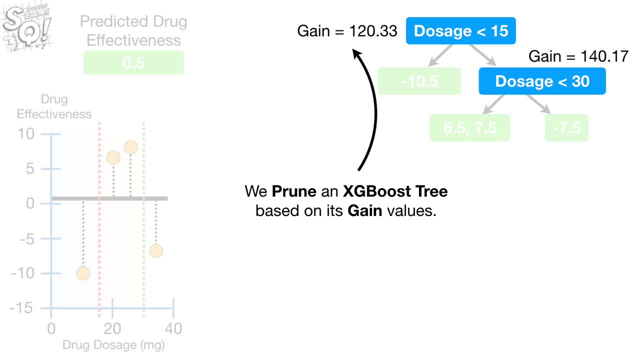 We prune an XGBoost tree based on its gain values. We start by picking a number, for example 130.. No, It's the dreaded terminology alert. XGBoost calls this number gamma. We then calculate the difference between the gain. 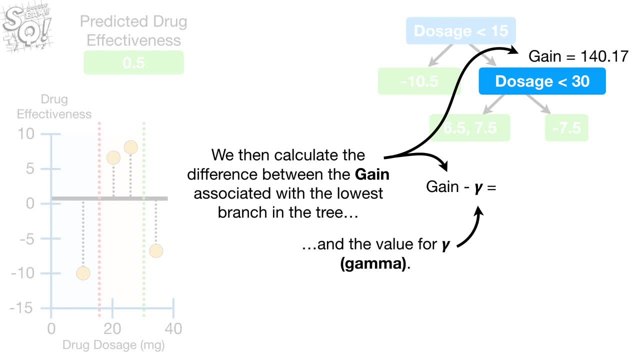 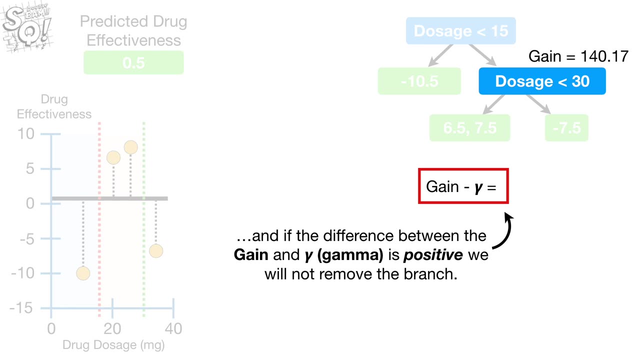 associated with the lowest branch in the tree and the value for gamma. If the difference between the gain and gamma is negative, we will remove the branch, And if the difference between the gain and gamma is positive, we will not remove the branch. In this case, when we plug in the gain. 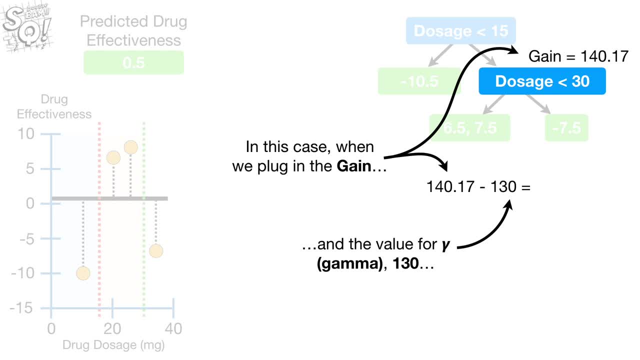 and the value for gamma 130, we get a positive number. so we will not remove this branch and we are done pruning. the gain for the root- 120.3, is less than 130, the value for gamma. so the difference will be negative. 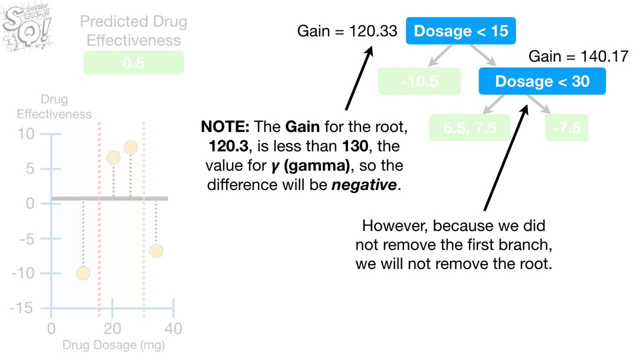 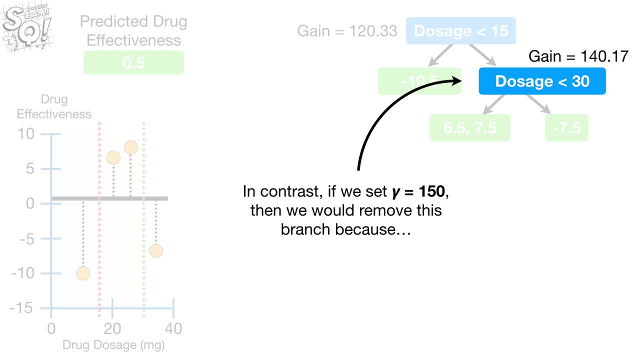 However, because we did not remove the first branch, we will not remove the root. In contrast, if we set gamma equal to 150, then we would remove this branch, because 140.17 minus 150 equals a negative number. So let's remove this branch. 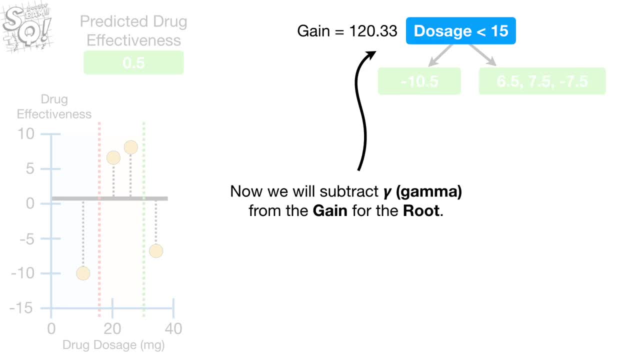 Now we subtract gamma from the gain for the root, Since 120.33 minus 150 equals a negative number, we will remove the root And all we would be left with is the original prediction, which is pretty extreme pruning. So, while this wasn't the most nuanced example, 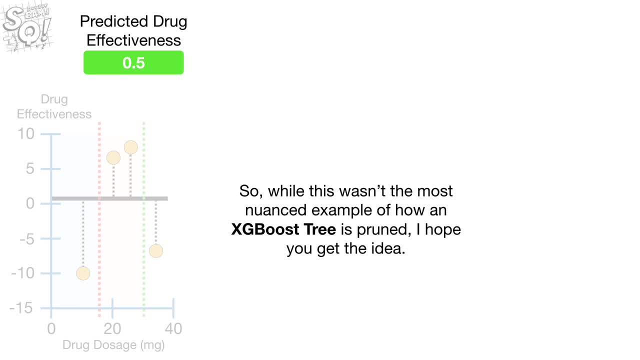 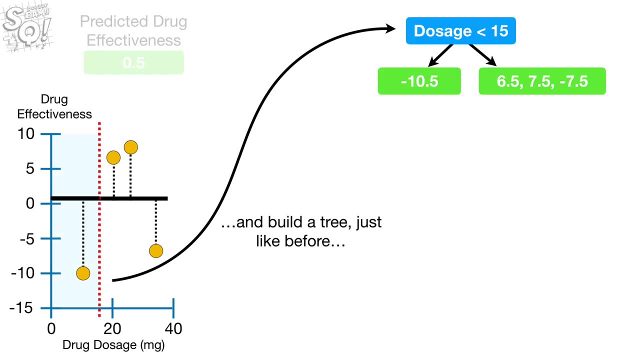 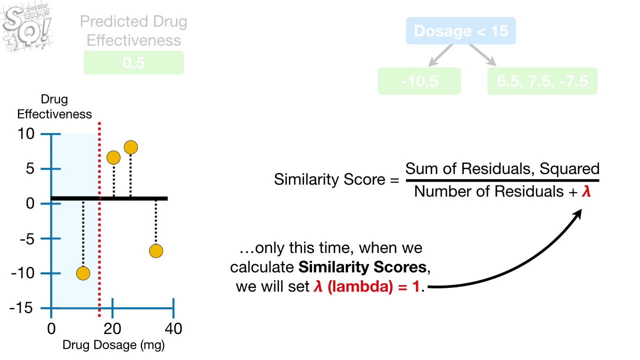 of how an XGBoost tree is pruned. I hope you get the idea. Now let's go back to the original residuals and build a tree just like before. only this time, when we calculate similarity scores, we will set lambda equal to 1.. 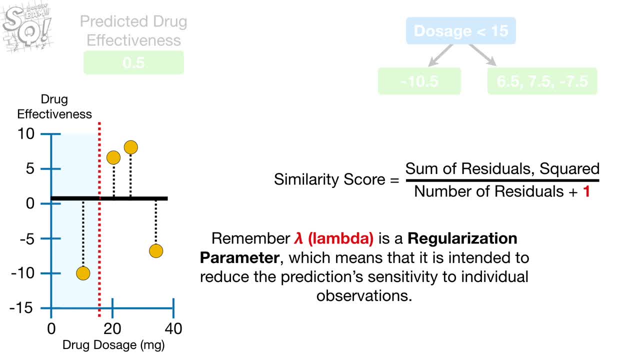 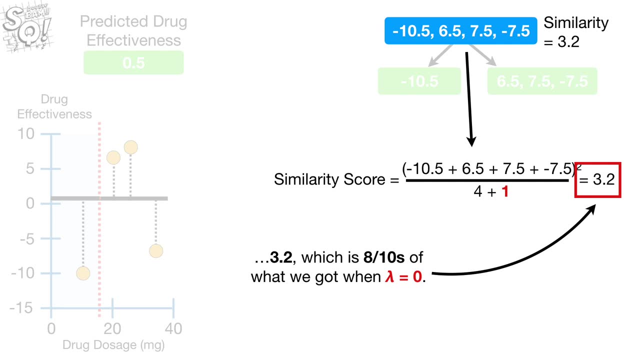 Remember, lambda is a regularization parameter, which means that it is intended to reduce the prediction sensitivity to individual observations. Now the similarity score for the root is 3.2, which is 8 tenths of what we got when lambda equals 0.. 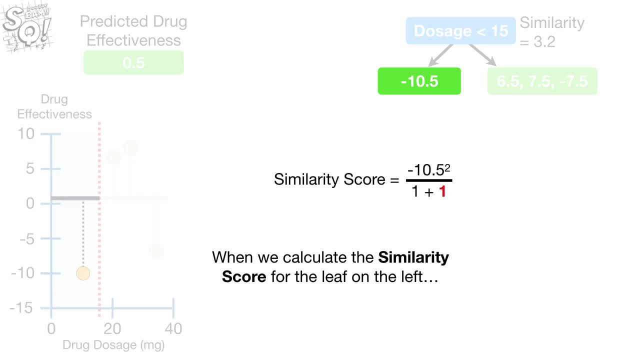 When we calculate the similarity score for the leaf on the left, we get 55.12,, which is half of what we got when lambda equals 0. And when we calculate the similarity score for the leaf on the right, we get 10.56, which is 3 quarters of what we got. 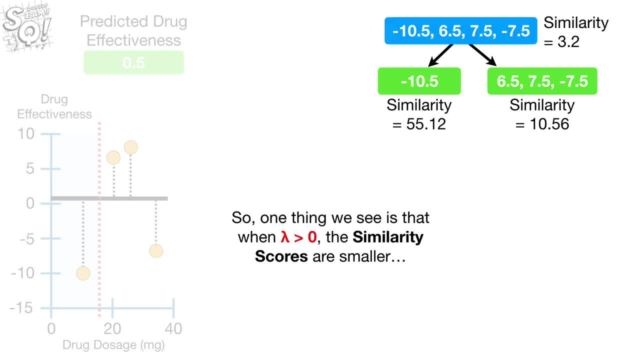 when lambda equals 0. So one thing we see is that when lambda is greater than 0, the similarity scores are smaller and the amount of decrease is inversely proportional to the number of residuals in the node, In other words, the leaf on the left. 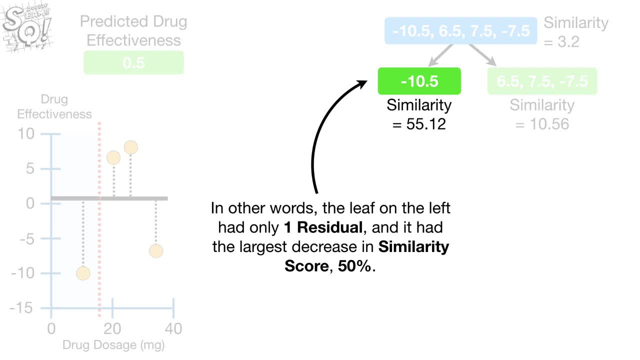 had only one residual and it had the largest decrease in similarity score: 50%. In contrast, the root had all four residuals and the smallest decrease: 20%. Now, when we calculate the gain, we get 66, which is a lot less than 120.33,. 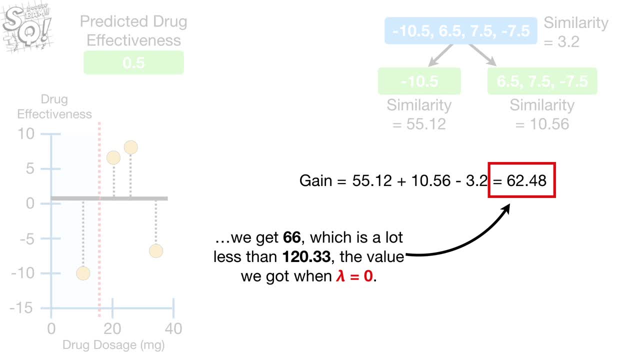 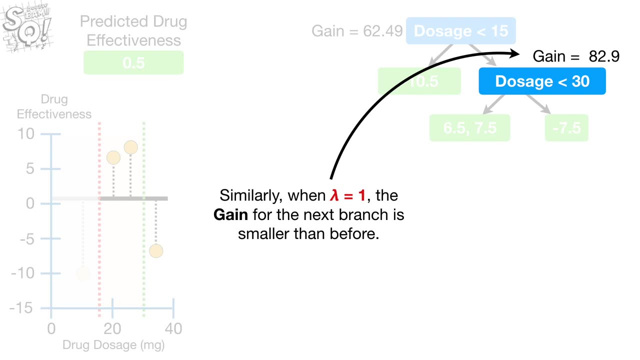 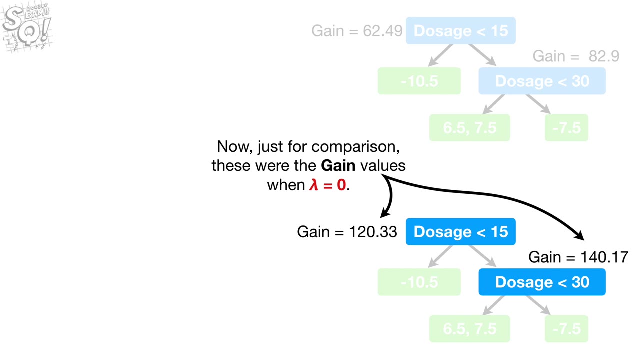 the value we got when lambda equals 0.. Similarly, when lambda equals 1, the gain for the next branch is smaller than before. Now, just for comparison, these were the gain values when lambda equals 0.. When we first talked about pruning trees, 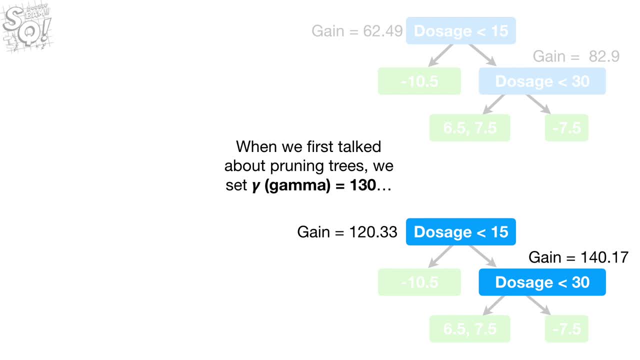 we set gamma equal to 130.. And because for the lowest branch in the first tree, gain minus gamma equaled a positive number, so we did not prune at all. Now, with lambda equals 1, the values for gain are both less than 130. 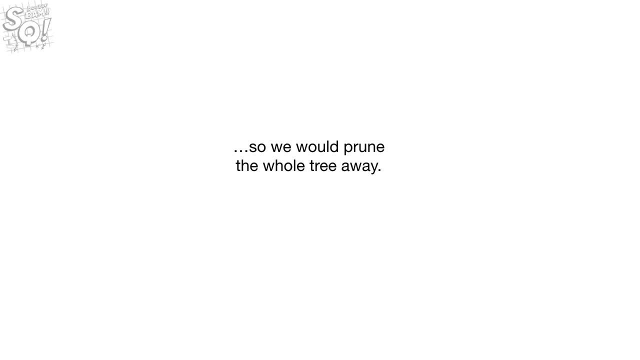 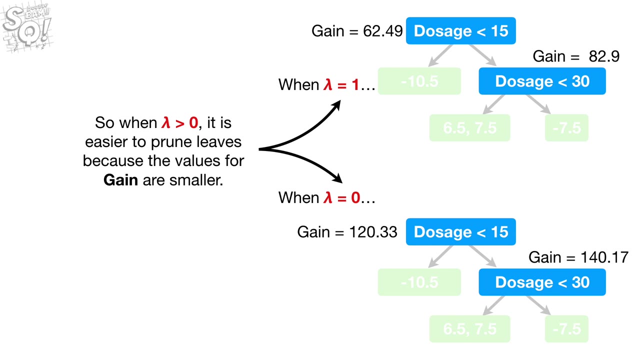 So we would prune the whole tree away. So when lambda is greater than 0, it is easier to prune leaves because the values for gain are smaller. Before we move on, I want to illustrate one last feature of lambda. For this example, 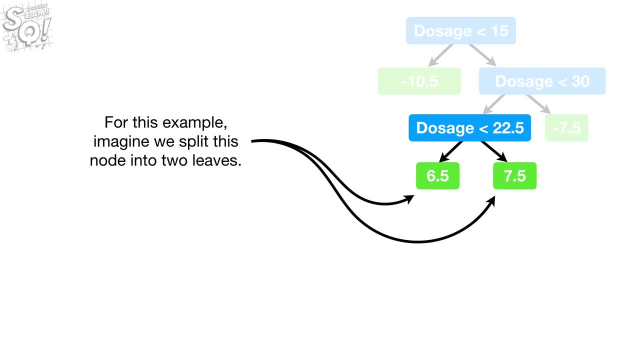 imagine we split this node into two leaves. Now let's calculate the similarity score with lambda equal to 1.. For the branch we get 65.3.. For the left leaf we get 21.12.. And for the right leaf we get 28.12.. 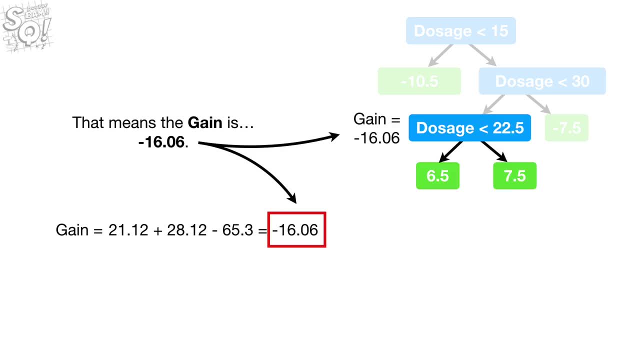 That means the gain is negative 16.06.. Now, when we decide if we should prune this branch, we plug in the gain and we plug in a value for gamma. if we set gamma equal to 0, then we will get a negative number. 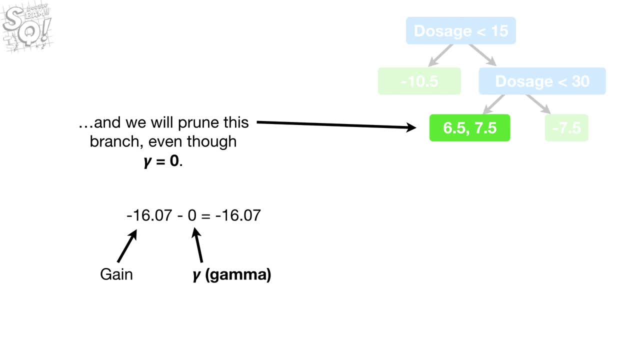 And we will prune this branch even though gamma equals 0. In other words, setting gamma equal to 0 does not turn off pruning Dang. On the other hand, by setting lambda equal to 1, lambda did what it was supposed to do. 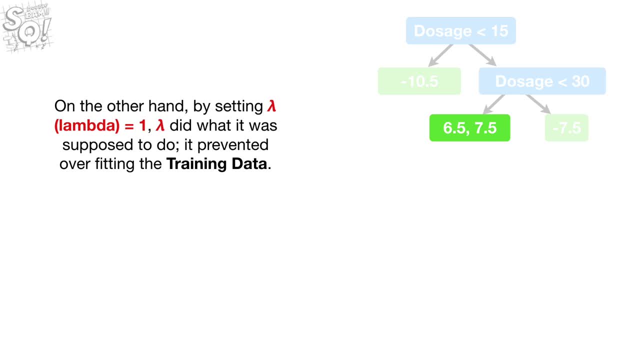 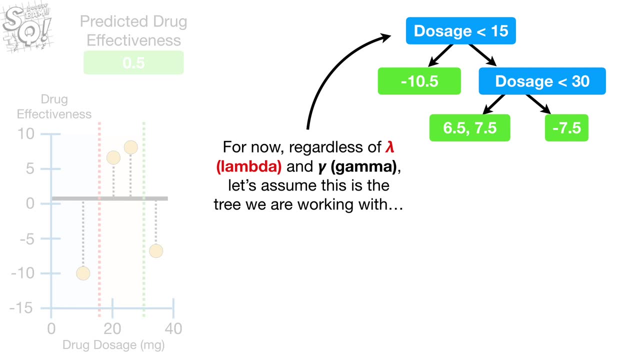 It prevented overfitting the training data. Awesome For now, regardless of lambda and gamma, let's assume that this is the tree we are working with and determine the output values for the leaves. The output value equals the sum of the residuals. 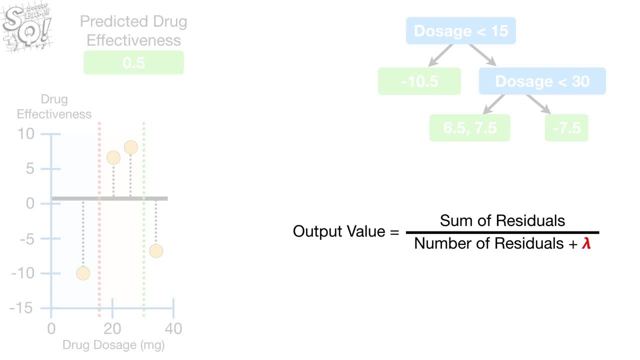 divided by the number of residuals plus lambda, the output value equation is like the similarity score, except we do not square the sum of the residuals. So for this leaf we plug in the residual negative 10.5, the number of residuals in the leaf: 1,. 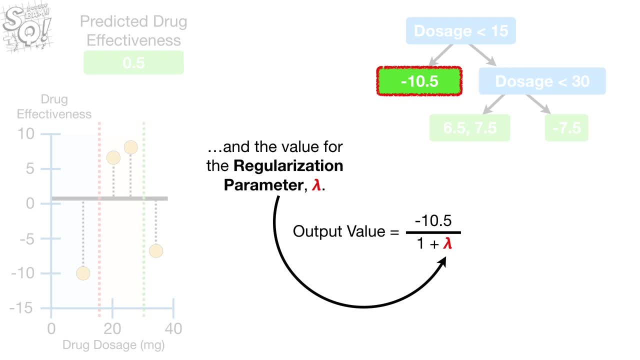 and the value for the regularization parameter lambda. If lambda equals 0,, then there is no regularization and the output value equals negative 10.5.. On the other hand, if lambda equals 1,, the output value equals negative 5.25.. 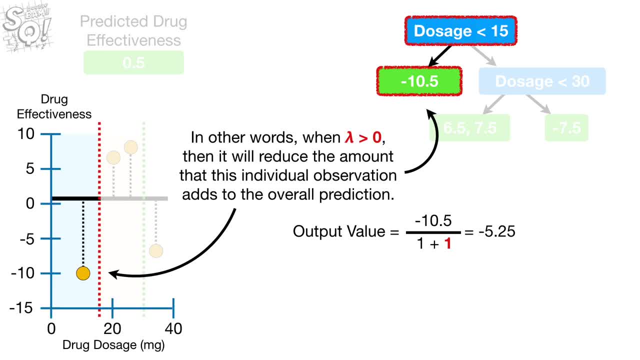 In other words, when lambda is greater than 0,, then it will reduce the amount that this individual observation adds to the overall prediction. Thus, lambda, the regularization parameter, will reduce the prediction sensitivity to this individual observation. For now, we'll keep things simple. 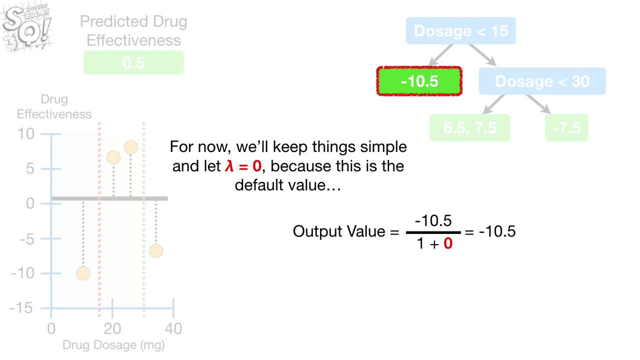 and let lambda equals 0,, because this is the default value, and put negative 10.5 under the leaf. so we will remember it. Now let's calculate the output value for this leaf. When lambda equals 0,, the output value is 7.. 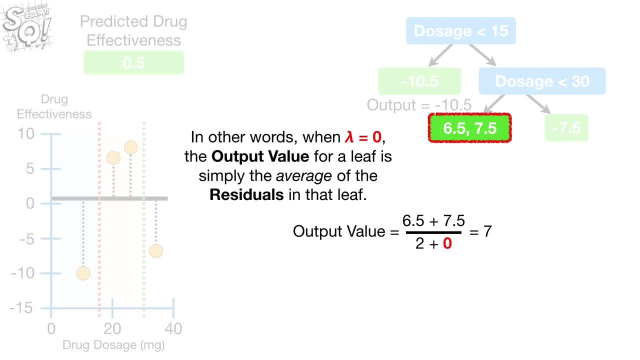 In other words, when lambda equals 0, the output value for a leaf is simply the average of the residuals in that leaf. So we'll put the output value under the leaf, so we will remember it. Lastly, when lambda equals 0,, 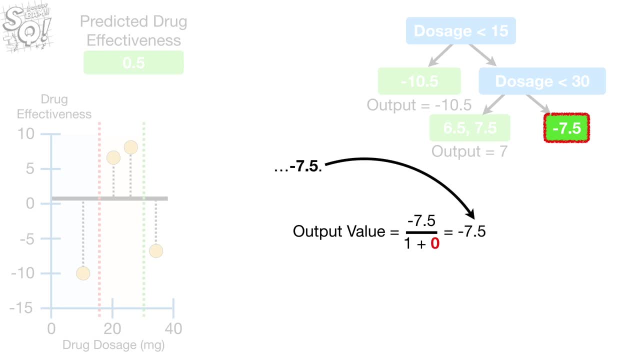 the output value for this leaf is negative 7.5.. Now, at long last, the first tree is complete Double BAM. Since we have built our first tree, we can make new predictions And, just like Unextreme Gradient Boost. 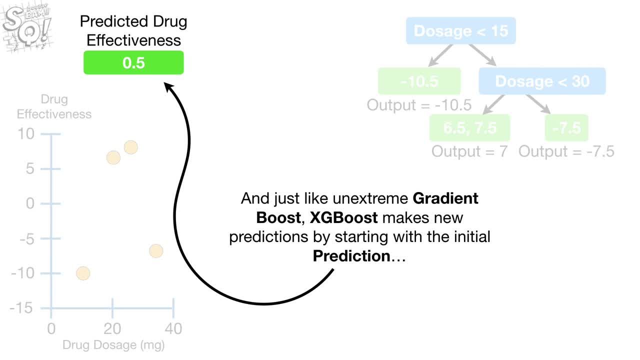 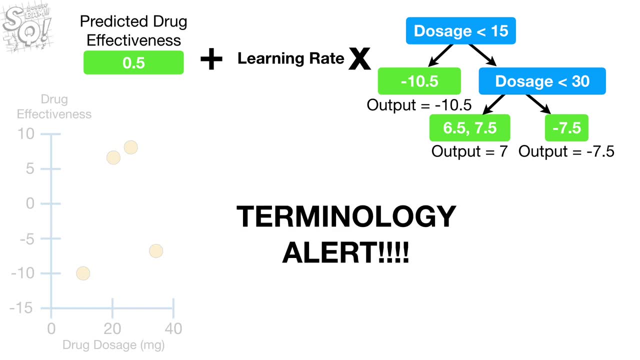 XGBoost makes new predictions by starting with the initial prediction and adding the output of the tree Scaled by a learning rate. Oh no, It's another dreaded terminology alert. XGBoost calls the learning rate eta and the default value is 0.3,. 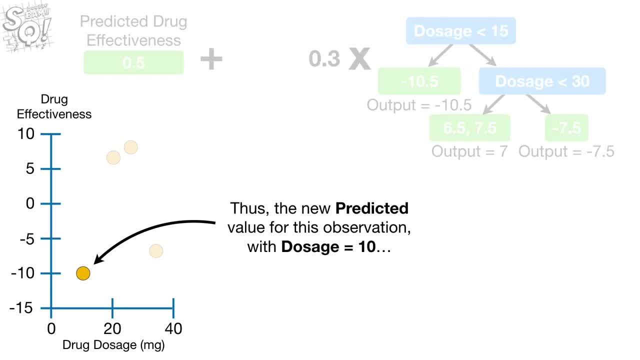 so that's what we'll use. Thus, the new predicted value for this observation with dosage equal to 10 is the original prediction: 0.5, plus the learning rate, eta 0.3, times the output value negative 10.5.. 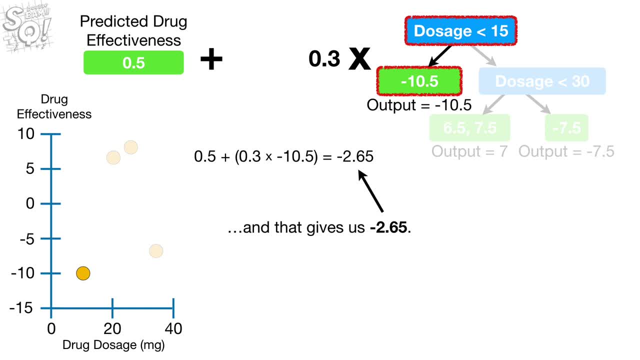 And that gives us negative 2.65.. So if the original prediction was 0.5,, then this was the original residual. The new prediction is negative 2.65, and we see that the new residual is smaller than before. 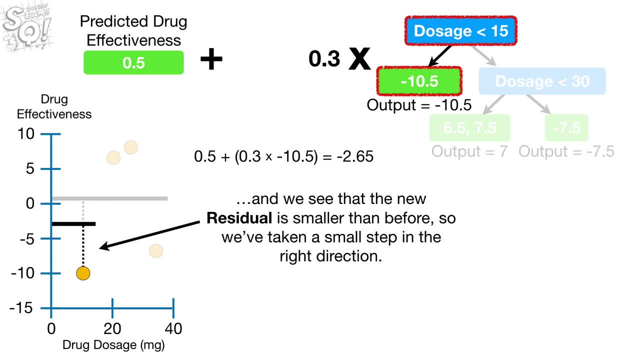 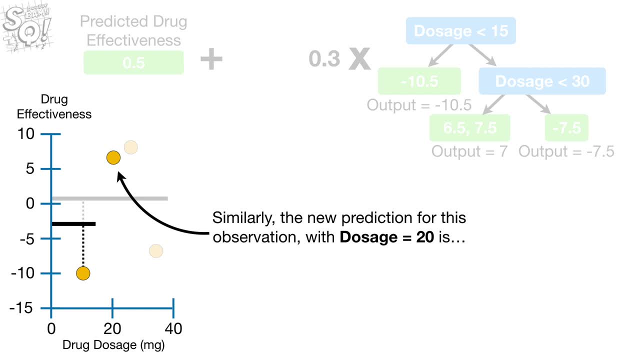 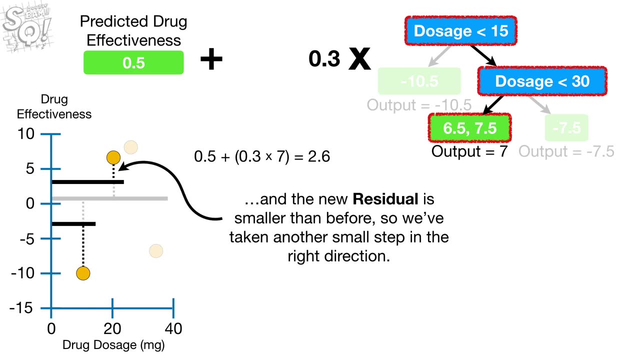 so we've taken a small step in the right direction. Similarly, the new prediction for this observation with dosage equal 20 is 2.6, and the new residual is smaller than before. so we've taken another small step in the right direction. 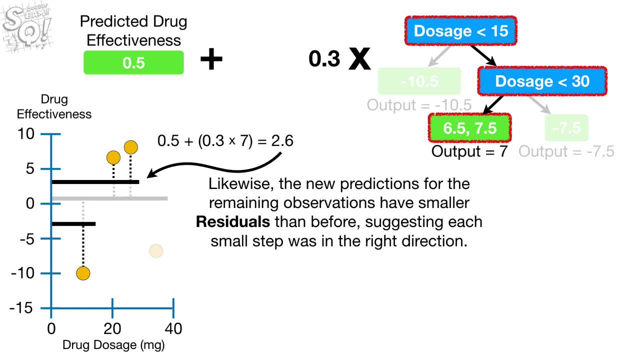 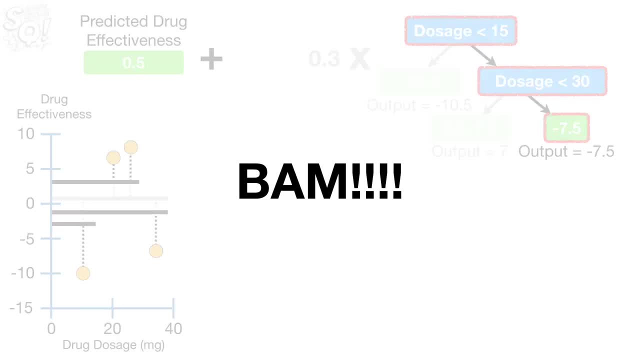 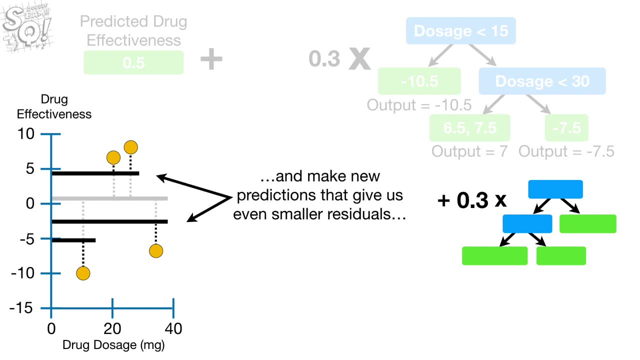 Likewise, the new predictions for the remaining observations have smaller residuals than before, suggesting each small step was in the right direction. Bam, Now we build another tree based on the new residuals and make new predictions that give us even smaller residuals, And then build another tree. 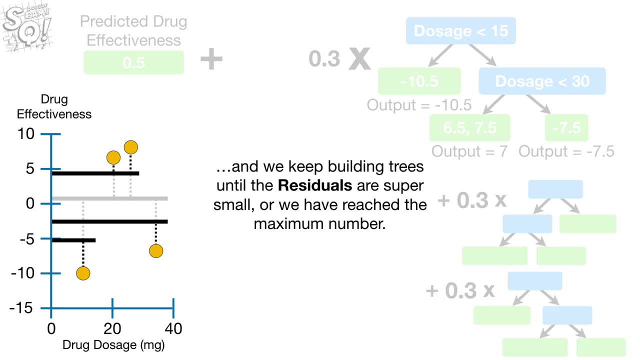 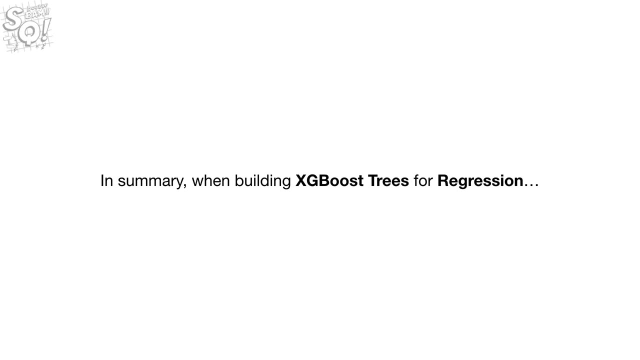 based on the newest residuals And we keep building trees until the residuals are super small or we have reached the maximum number. Triple bam. In summary, when building XGBoost trees for regression, we calculate similarity scores and gain to determine how to split the data.